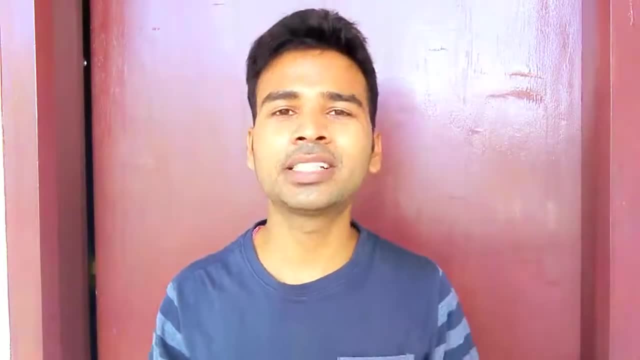 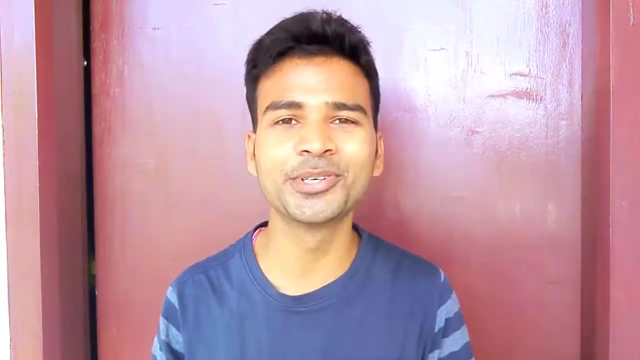 Hey, what's up guys. This is Abhishek here, and welcome back to my channel, Technical Tech. This is another episode on IP address, and in today's video I am going to show you how to sort your IP version 6 address. 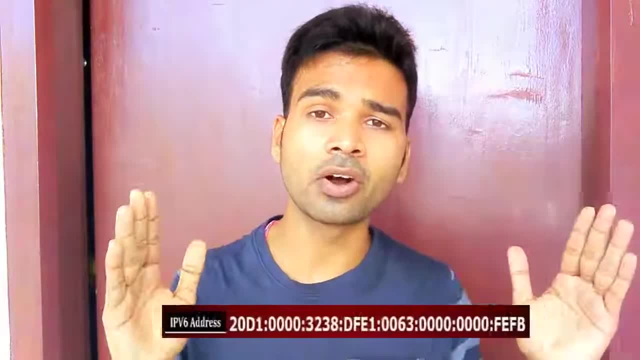 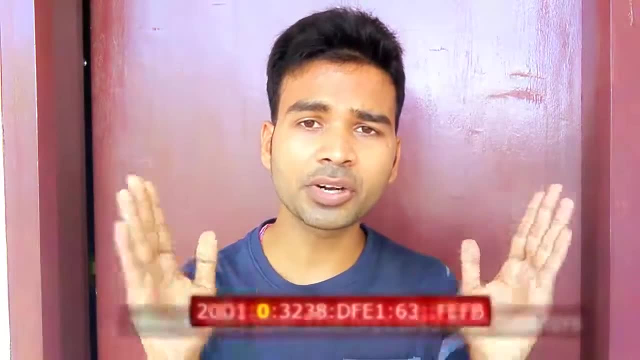 Guys, you have noticed that IP version 6 addresses are quite long. okay, But in today's video I am going to show you few easy steps. with the help of that you can sort your IP version 6 address, okay. So what are these tricks? Let's find out. 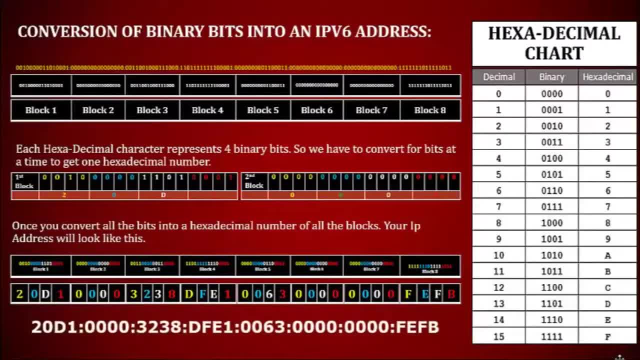 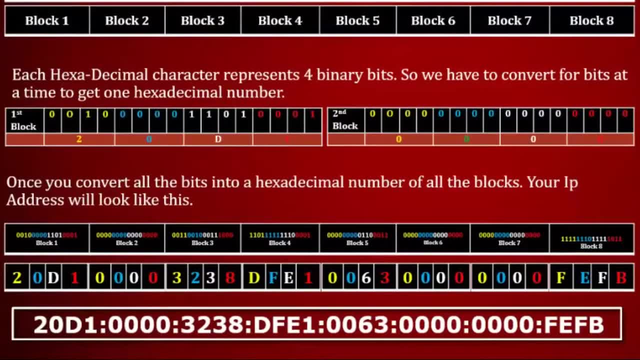 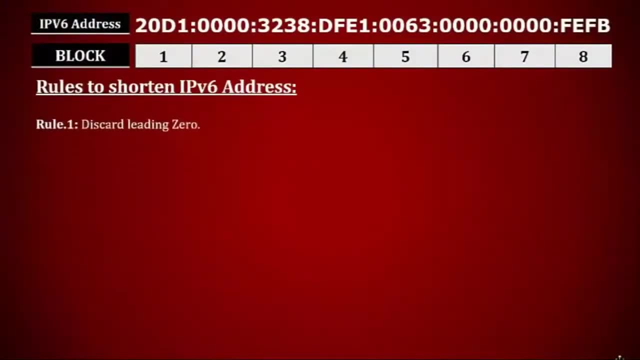 This address is too long and it is very difficult to remember and write. So we are having some rules using which you can make this IP address short and simple. So, guys, let's find these rules. Rule number 1. Discard leading zeros. 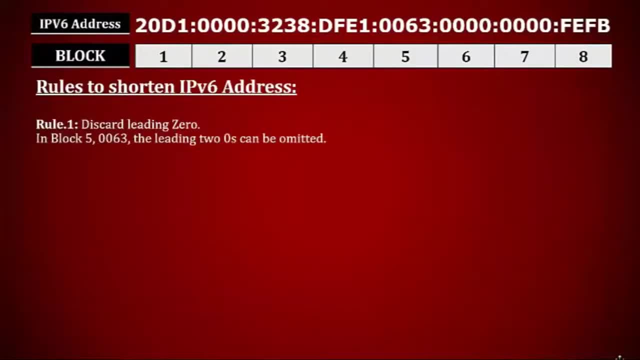 Which means if you see any zero at the starting of each block, you can discard it. As, for example, you can see in block 5, we are having two leading zeros, so you can discard this zero. and now, once you discard this zero, your IP address will look like this: 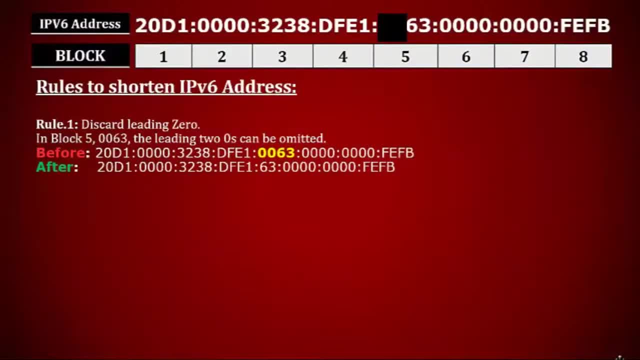 Still the IP address looking too long. So the rule number 2 is: if two or more blocks contain consecutive zeros, omit them all and replace with double colon sign, Which means if you find two blocks too long, you can discard them. 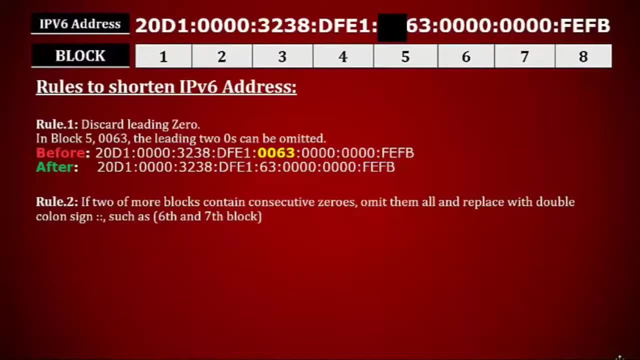 Which means if you find two blocks too long, you can discard them all and replace with double colon sign. Which means if you find two blocks too long, just we need to delete the blocks together containingna all key zeros. Then it can omit and replace them with double colon sign. 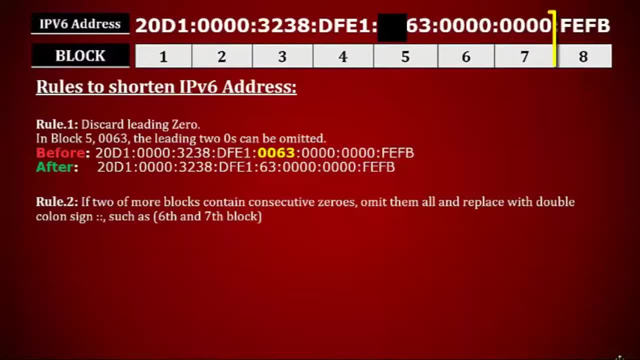 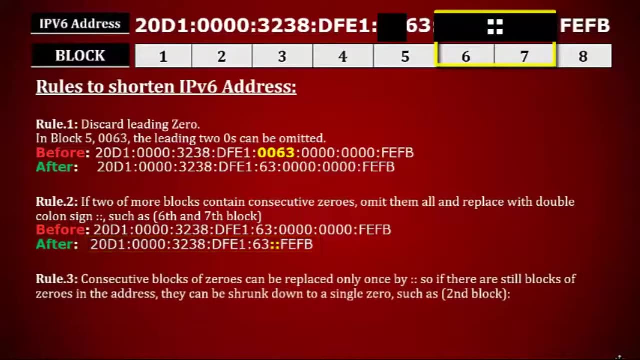 As for example here we can see 6th and 7th blocks are containing consecutive zeros, So we are going omit this zeros and replace it with double colon sign. Now IP address will look like this: Rule number 3 is: consecutive block of zeros can be replaced only once by double colon sign. 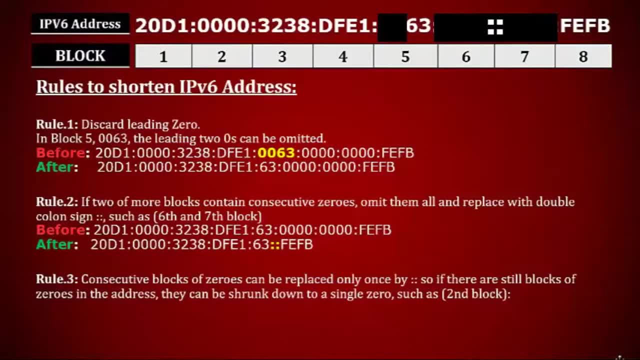 Rule number 3 is: consecutive block of zeros can be replaced only once by double colon sign. So if there are still blocks which contains only zero in the address, they can be shrunk down to a single zero, which means if there is still blocks containing only zero, it can.